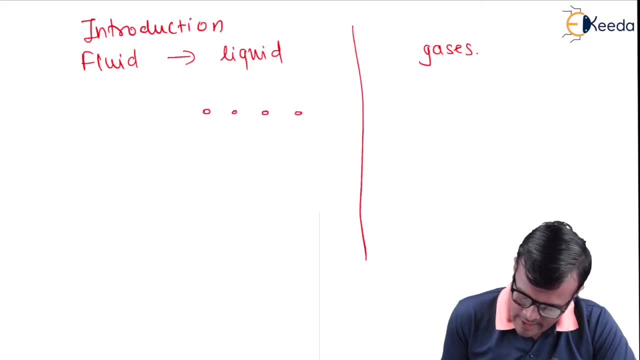 molecules is closer, as seen in figure, when compared with arrangement in gases like this. so it means that there exists spaces between gases as compared to the liquid. so it is clear that if I want to compress a particular fluid, if it is liquid then it will get slightly compressed, and if it is gas it will get. 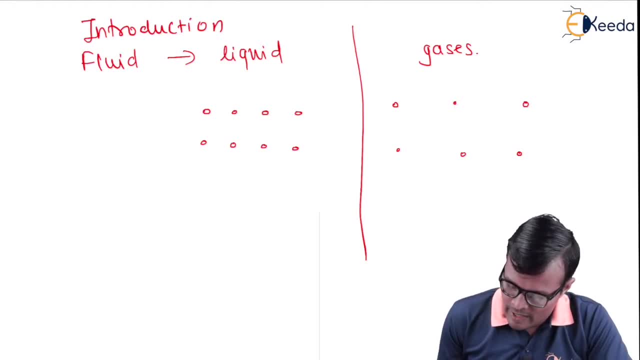 compressed in large amount. so actual compression process referred as shown in figure here. after compression molecules will get compactly packed into the gases. so this is the reason why gases becomes liquid after compression. we know in day-to-day life there exists a butane gas which is filled into the cylinder in domestic use. 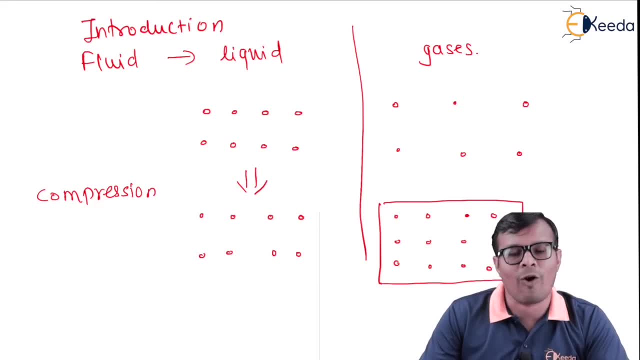 which is in liquid format. it is because it is compressed at high pressures so it makes changes in the stages from gases to liquid. so it is clear that if I talk about compression capacity, liquid have very less or very negligible compressive compression capacity. for water we generally say that it is ideal fluid, so it is incompressible. 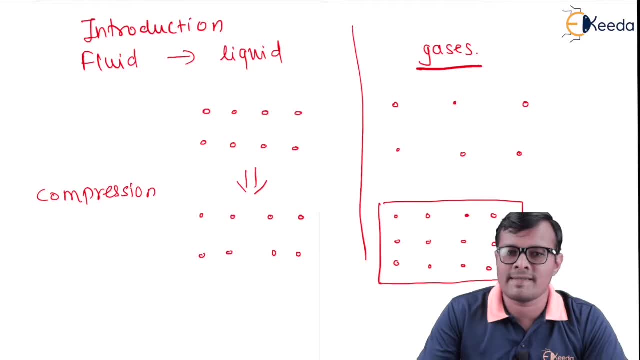 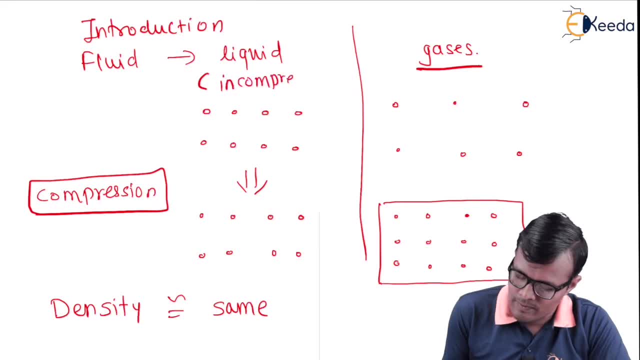 so we call liquid as incompressible. in case of gases, this density changes, actually increases. so in this case increase in density is same when we do the process of compression. in case of gases it is obvious because if I want to define density, density is nothing but the ratio of mass per unit volume. imagine that we have a 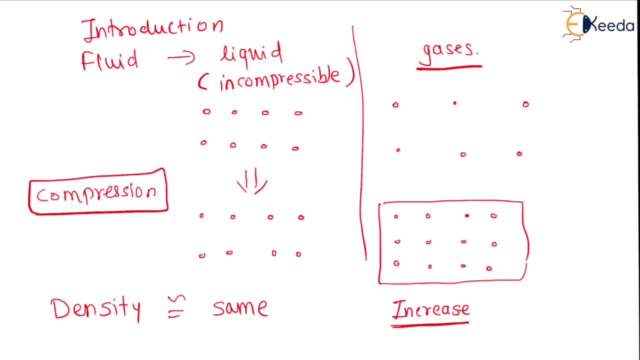 cube having dimensions of unity, say for example one meter length, one meter wide and one meter height. so in this cube if I feel liquid, then whatever will be the mass situated in that volume is called as density. so generally in one meter cube 1000 kg of water is filled, hence the density changes. 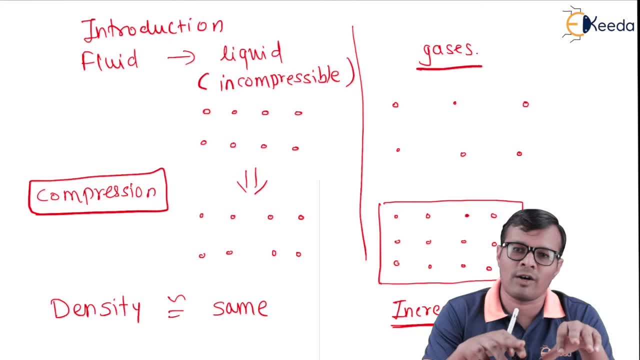 the density of liquid is 1000 kg per meter cube. if we talk about air, it is something 1.2 kg or 1 kg something. so it is. when compared with liquid it is very, very less. but if I do a compressor, if I do the process of compression in case of liquids, then in that case more. 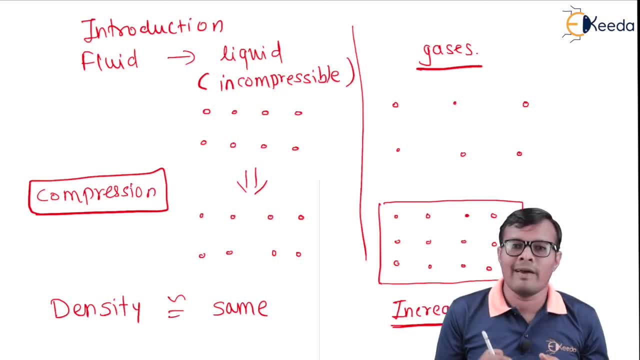 molecules will get accommodated in one meter cube. hence its self-wet is going to increase in the same amount of volume. it means that its density is going to increase. so this is the reason. compression is the reason which increases the density of gas in fluid mechanics. 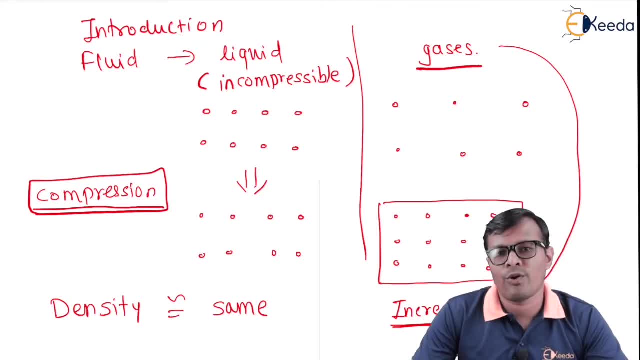 we generally consider two types of densities. we should know the basic values of densities, say, for example, if I talk about density, density may be defined as mass per unit volume. it can be divided into two types: either mass density or mass per unit volume. mass density is expressed in kg per meter cube, which is 1000 for water weight as its name. 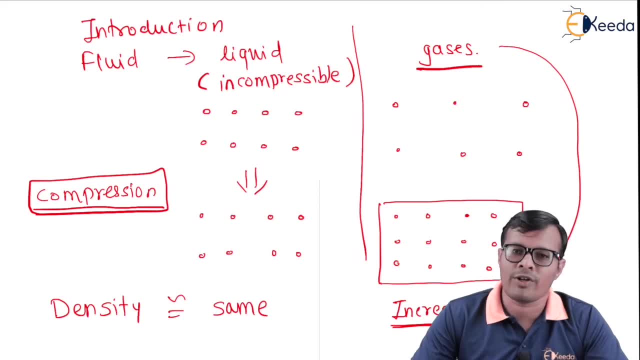 indicate it is expressed in Newton or kilonewton, and its unit is Newton per meter cube or kilonewton per meter cube, and its value is 9810 Newton per meter cube for water or 9.81 kilonewton per meter cube for water. 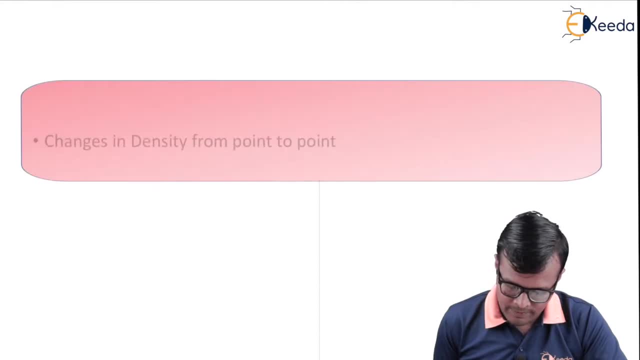 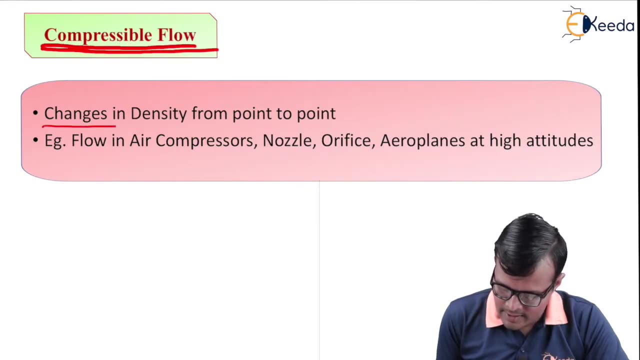 So let us start with actual topic: incompressible flows. changes in the density from point to point are occurred. so the type of flow in which we can see the changes in the density, we can say the flow is compressible. this is the very simple definition of compressible. 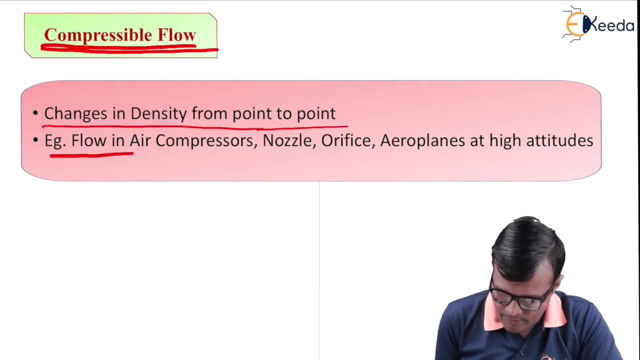 flow. What is a flow in air compressor? we all know that compressor is the thing which compresses the air, hence called as compressor. actually, there exists a pump. this is cylinder, in which this is the piston. this is rotated by means of a crankshaft And this is the rotation, say clockwise rotation, so clockwise rotation of any source. so this: 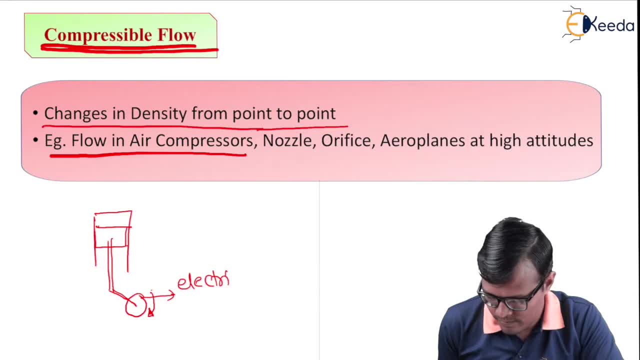 source may be either electric motor or diesel engine or any source which can rotate. so rotation of crankshaft moves piston in upward and downward direction And there exists a non return wall which is very important. This is non return wall. non return wall which operates in only one direction. it means that 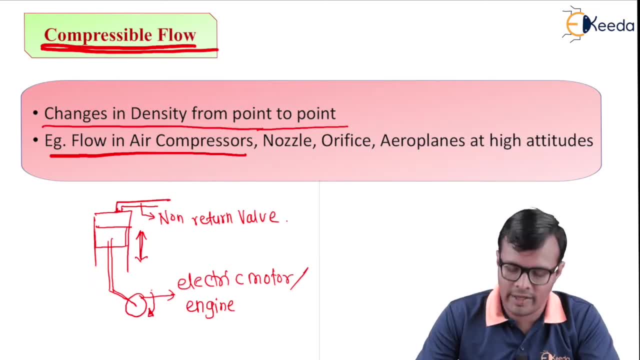 it allows a unidirectional flow of water or flow of liquid or flow of fluid that may be air. So this non return wall allows the air to come in. What are the references? another non-written wall allows the air- compressed air- to go out. so simultaneous actions of both the 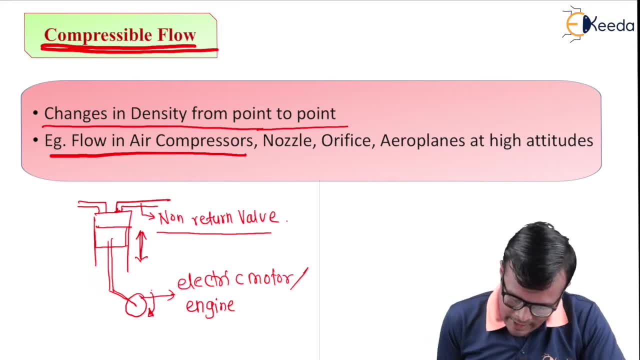 walls compresses the air and they are temporarily stored into a cylinder or tank in compressed format. we have a pressure gauge located over the tank and on pressure which we can say what is the pressure actually currently. so this tank actually for saving compressed air and this compressed air. 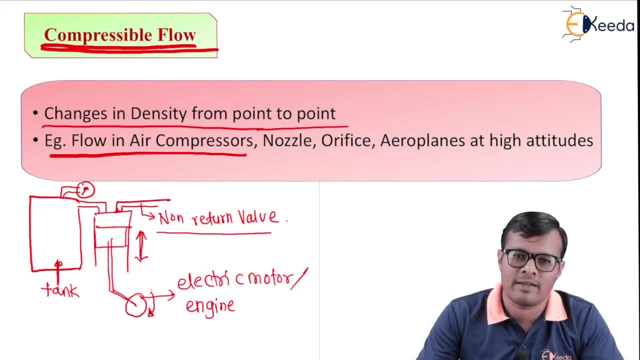 is then after used wherever it is necessary. we know in various styles we fill up the air by using this compressor. so this is the day-to-day life example in which density of air is continuously changing. in piston, actual density is different. when it comes at compressor, actual density is different. so flow of air in compressor. 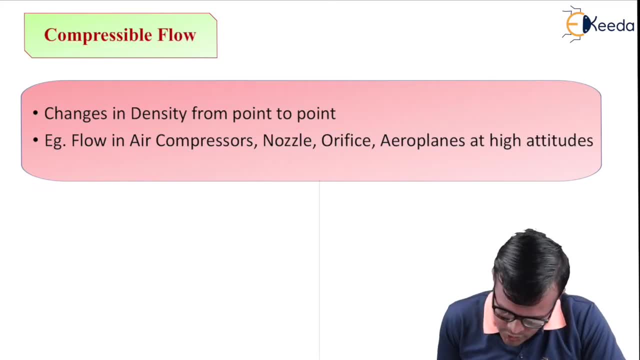 is the example of compressible flow. so in case of nozzle there exists a pipe, its cross section is get reduced with respect to length up to certain dia. this is initial dia d after compression. small dia b, small d: this is small dia, this is large dia d. so when we trace flow of air particles, say, for example, these are the air particles. 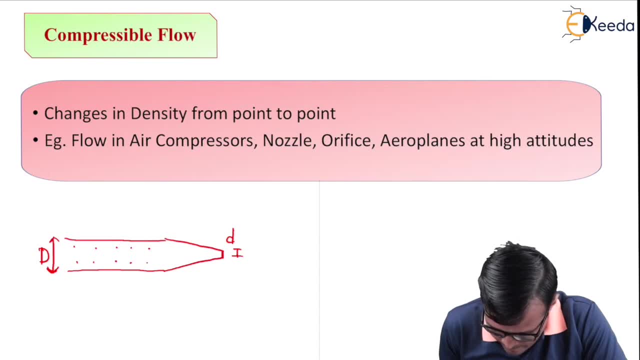 in normal dia these, when traveled through the section of nozzle, these particles get closer to each other. if particles are get closer, it that its density is increased. this is the example of compressible flow. it means that now particles are get compressed. so this is the example of 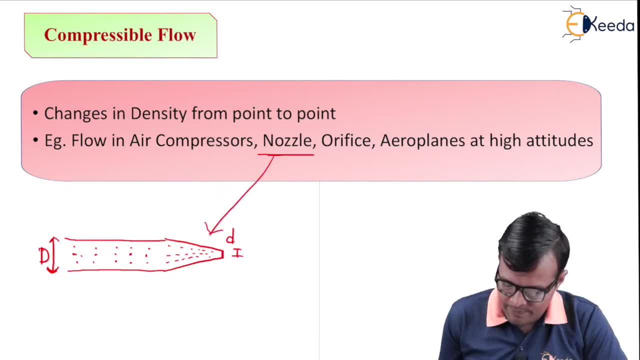 nozzle is the example of compressible flow. if I want to talk about orifice, orifice is nothing but a aperture which is provided in either tank or in liquid or in pipe. so say, for example, this is the pipe. to give rough idea, I am drawing a regular type of orifice. this orifice is formed by providing a disc having an 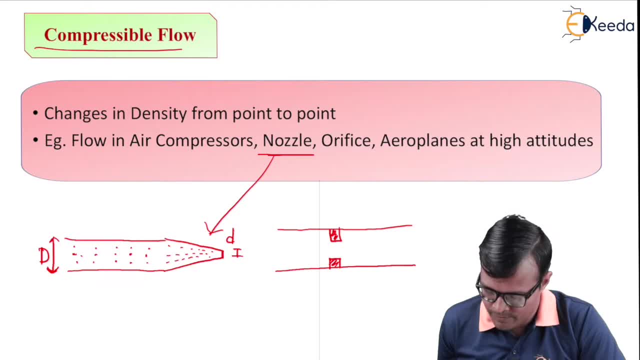 aperture and fitting that disc into the pipe cross-section. so in this case actual flow of particles is shown in this picture and dotted line. and again it is clear that the density of particles at the section of orifice is again increased. so this is the zone where 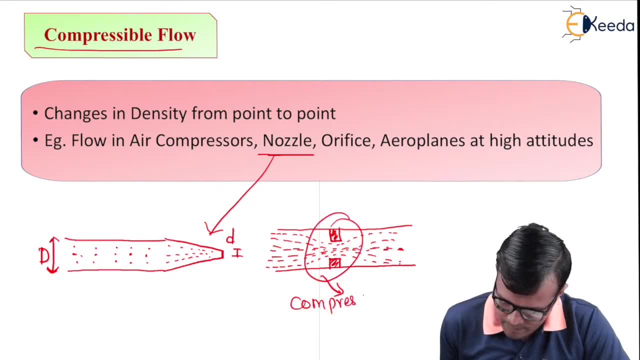 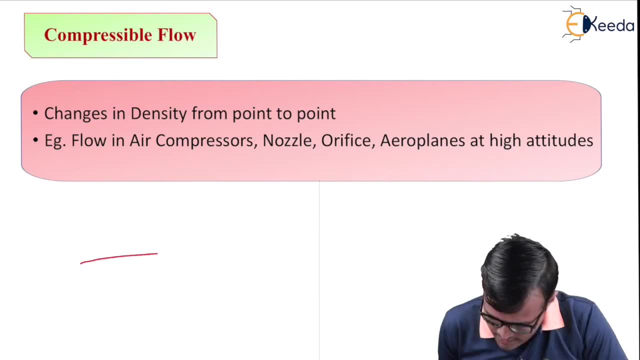 compression is occurring. so this is the example, orifice is the example of compressible flow flow. this is say, for example, an aeroplane having its wings like this. it's moving in this direction. so I will call this part as nose and this part as tail. we know that aeroplane moves in the forward direction by throwing out gases. 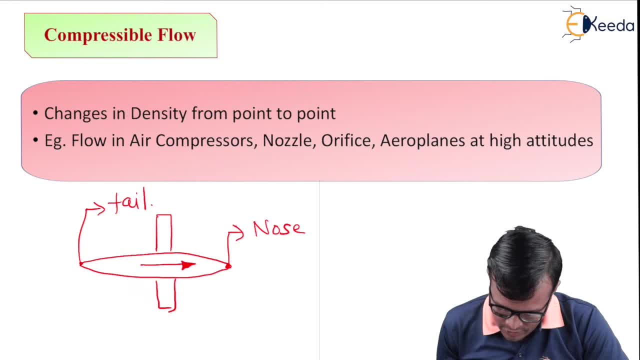 at very high speed. so that is the jet action. so gases are thrown out with very high speed from very reduced nozzle like aperture. so this is the first case where compression of air is okay and second case when streamlined shape, this type of shape, this type of shape of aeroplane, is called as streamlined, when 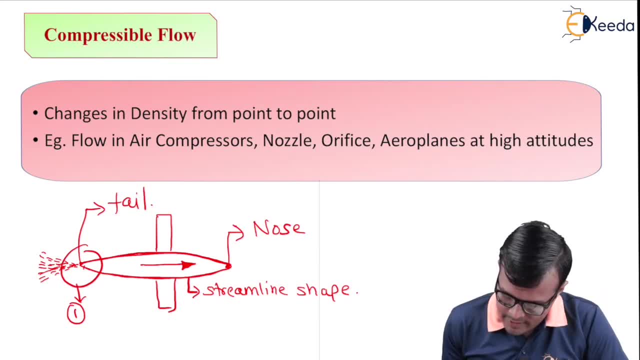 streamlined shape of aeroplane travels through normal particles, say. these are the air particles arranged normally. this is normal arrangement. so when through this media streamlined shape is traveling, it is nothing but replacing the particles in its path. so the particles which are located in the section of these nodes are nothing in the compressed stage. so this 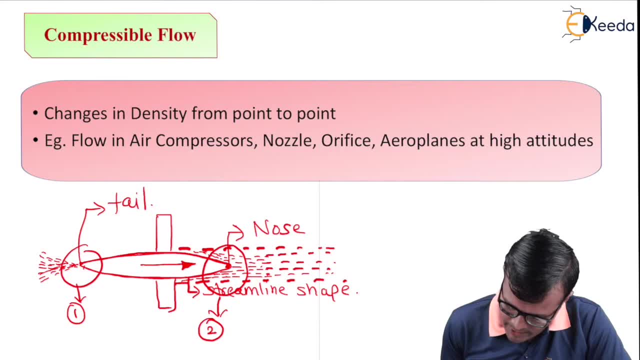 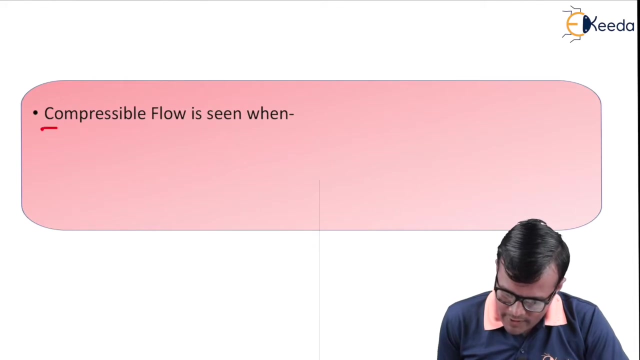 is. second is the example. second place is the example of compressible flow. so aeroplanes, each and every part of aeroplane which is replacing particles of air, is example, is best example of compressible flows. compressible flow is seen when first gas moving with high velocities, example. 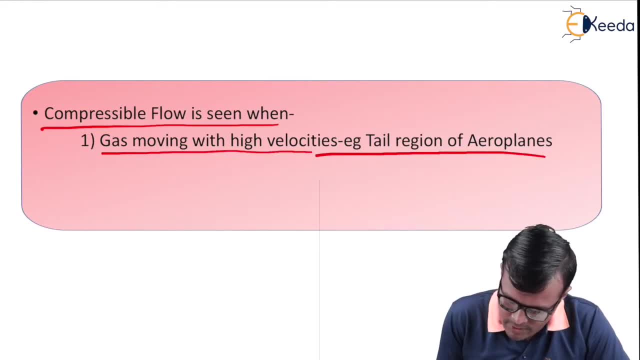 L region of aeroplane say, for example, this is aeroplane, this is the direction. so in this zone the compressed air is seen when gas is moving. so this is the case. first case, this is the case of gas moving with high velocities. it is also seen when 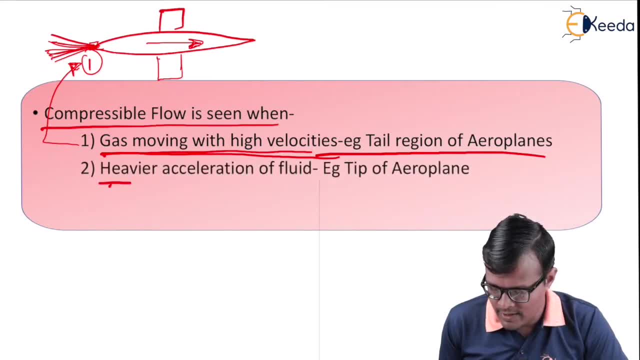 heavier acceleration of fluid. heavier acceleration of fluid means same is the aeroplane moving in this direction. so the acceleration of this particle in any other direction due to replacement of its place by aeroplane body, this, these particles try to move in the direction I am. 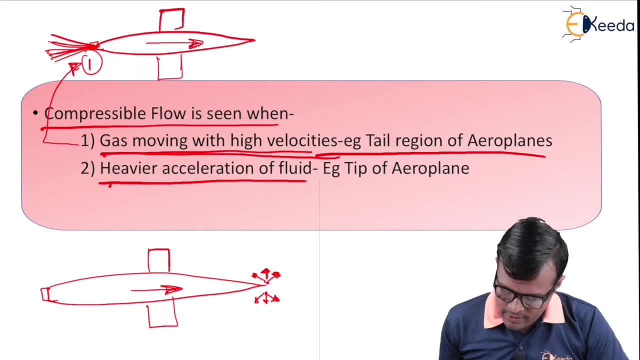 sure in the figure. so here, heavier acceleration, this is heavier acceleration of the fluid example type of aeroplane. so these are the places where compressible flow is seen. when there is a great change in elevation, large volume changes occur. we know that. density of air- if I want to talk about air density, it 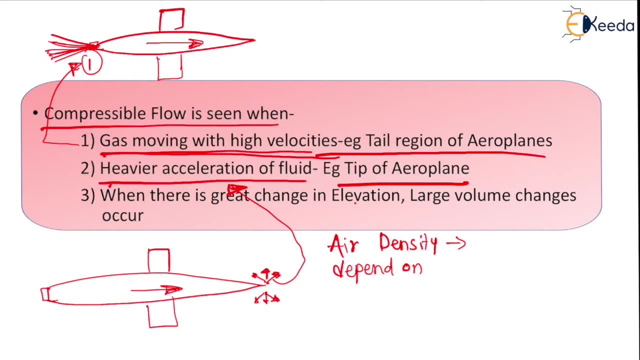 depends on elevation. it depends on elevation, say, for example, this is earth, this is our India, something like this. so this is everest if I see it from the point of view of the earth side view. this is everest side view. this is everest. so this is everest if I. 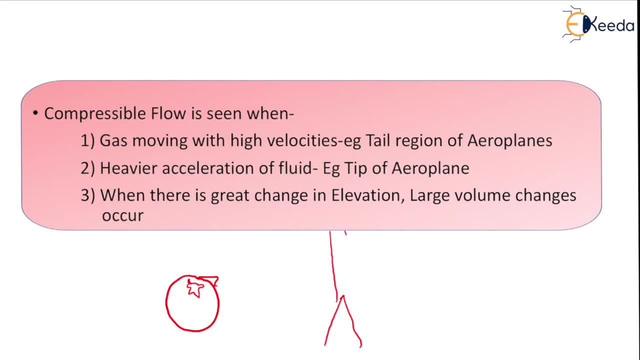 at the tip of over West as well as this is Mumbai, this is location of Mumbai. we know that Mumbai is located in the air. see I compare the same with respect to the Mumbai, then it is clear that there exist more amount of air particles due to height, that is, due to elevation. 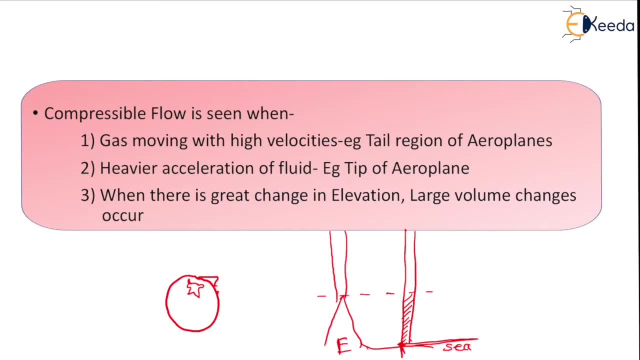 so this is everest, this is mumbai and if i talk about air column, the air column at everest is definitely having less height when compared with air column at mumbai. so the amount of air which is causing pressure, which is causing intensity of pressure, is more in mumbai, is when compared. 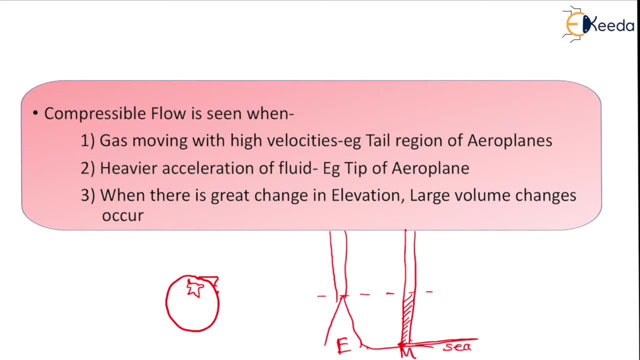 with everest. so we will find that particles at mumbai will get compressed properly when compared with particles at everest. so when a flight travels in this zone, when this flight travels like this, and when a flight travels like this in this direction, then densities suffered by the flight are different. 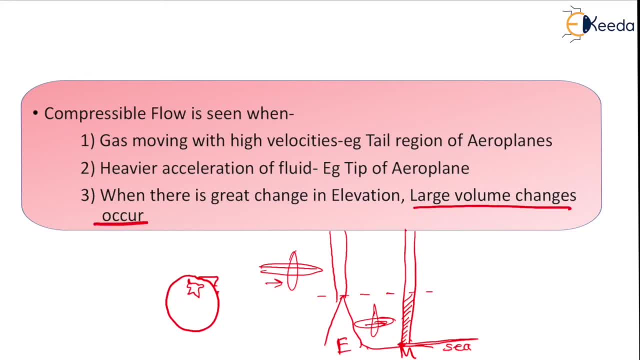 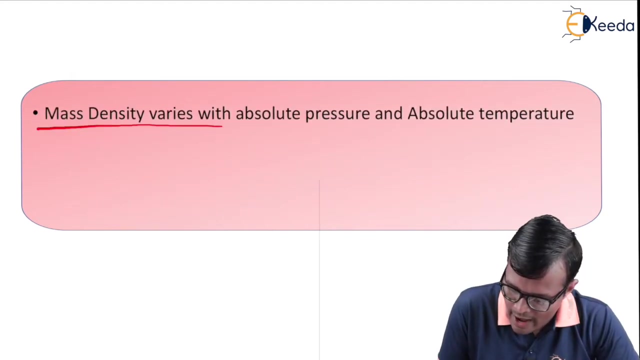 so large volume changes occur when there is a great change in elevation. so volume changes are occurred in these two examples. this is first and this is second. so volume change is the basic reason for compressible force. mass density varies with absolute pressure and absolute temperature. now i want to explain two. 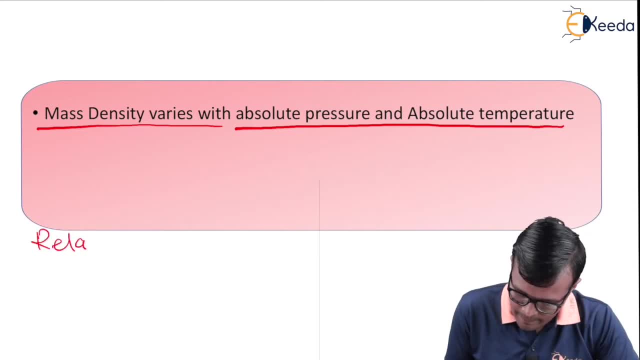 terms, relative and absolute. we know generally room temperature is 35 degree, so 35 degree is room temperature for 4 dick. when this range is the maximum heat downloaded during passage, this range increases the total temperature and the maximum heat is taken on basic線 and 35 degrees afterwards affects temperature. 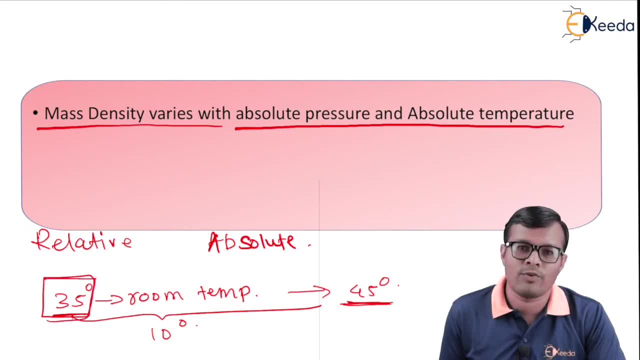 is relative temperature, with 0 degree centigrade, and this 45 degree is relative temperature with 0, with this 0 degree when compared with 0 degree. but when i want to compare 35 degree and 45 degree, this 10 degree is relative increase in the temperature when we compare with 35 degree. 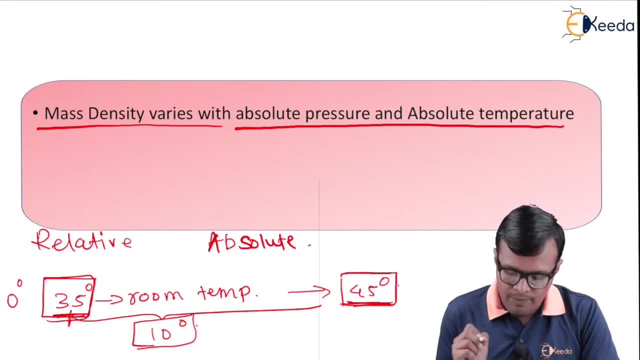 so in this case benchmark is set to zero. so this benchmark is depend on us. if i want to do scientific study in the subjects like thermodynamics, then we consider absolute zero temperature. but absolute zero temperature is not zero degree, but zero degree kelvin and relation between degree centigrade and kelvin is: 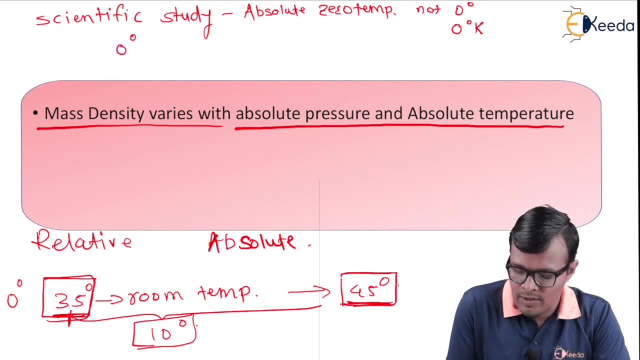 that zero degree plus 273.15 becomes 273.15 kelvin. so if i consider, when compared with zero degree centigrade minus 273.15 degree centigrade is called as absolute zero temperature. similar is the case when i talk about pressure. i was talking about temperature. so 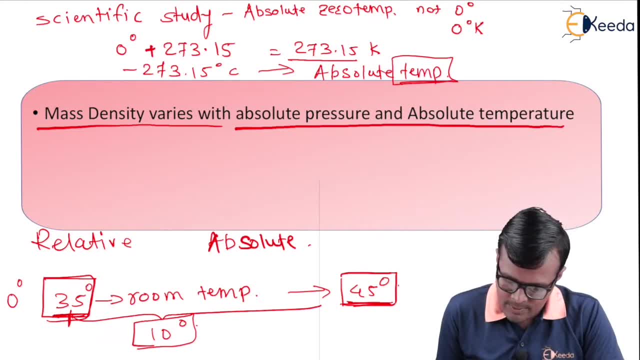 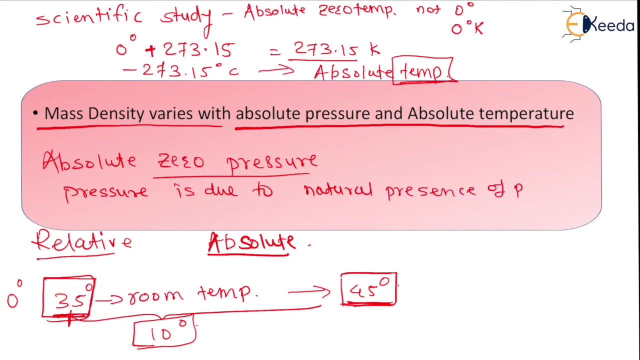 this was only the example to tell the concept of relative and absolute temperature. similar is the case with pressure. absolute zero pressure is the stage is the stage when pressure is due to natural presence of particles, stickty, so so on, at and JAC. 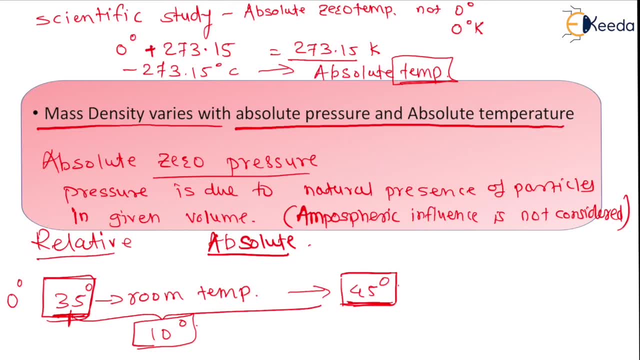 V V. talking about normal pressure, that is, pressure available in current situation, then it is clear that there exists atmospheric pressure in every situation. If we reduce that atmospheric pressure, then we will reach to the absolute zero pressure condition and that condition is considered. 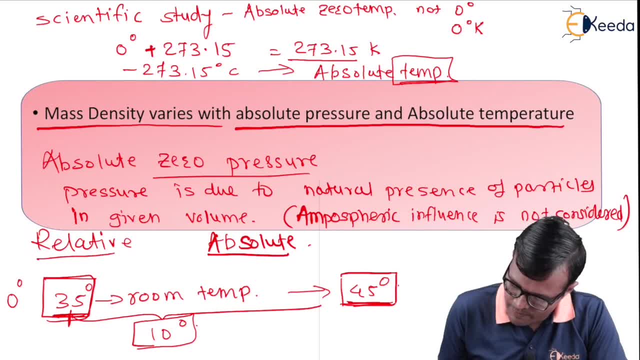 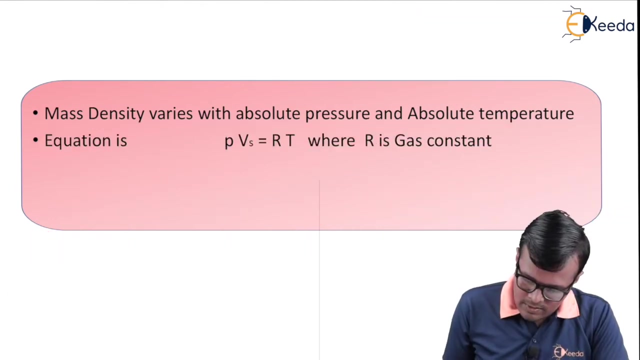 absolute zero pressure condition. So generally, at atmospheric height, at atmospheric situation, pressure is not zero. Which pressure? Absolute pressure. Okay, This was enough about the conditions: absolute temperature and absolute pressure. The general equation for perfect gas, the relation is P into four. 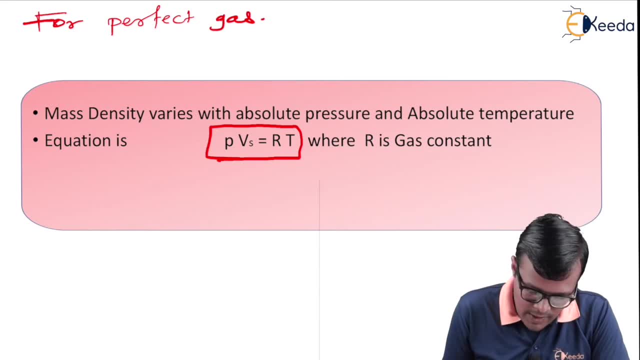 Vs is equal to R into T, where P is nothing but the pressure. V is specific volume. We know density is equal to mass upon volume. So specific volume is volume upon mass. Its unit is kg per meter cube and this is having unit meter cube per kg. 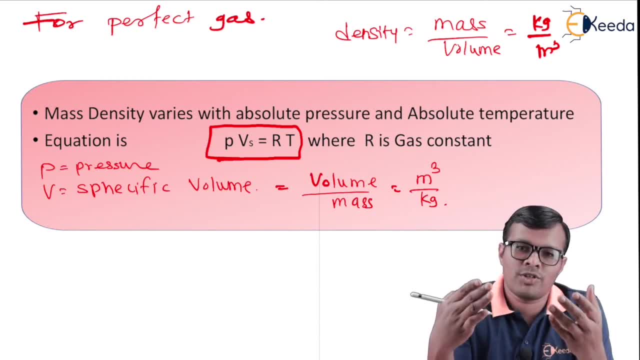 So if I want to talk about 1 kg gas, say 1 kg oxygen, Then how much volume it will take to occupy 1 kg of oxygen is called as that volume is called as R is called as gas constant. Some constants are defined in gases, in thermodynamics, so R is called as a constant term which does 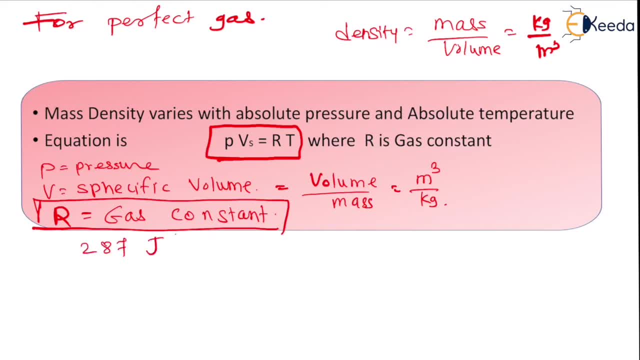 not change, Which is having value equal to 280.. is 7 joule per kg into kelvin. for hydrogen, its value is 4110 joules per kg into kelvin and t is nothing but the temperature. but the condition is that temperature should be expressed.